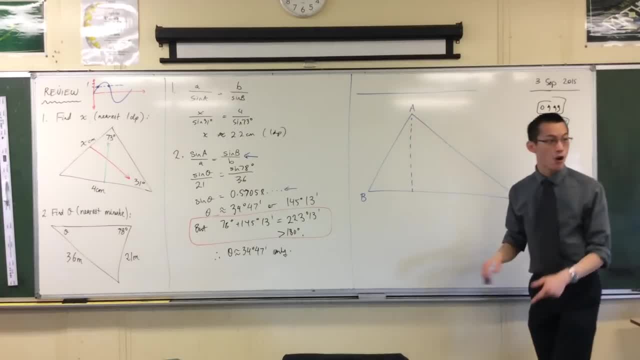 It's not right angled, so, in order to use the trigonometry that I know at the moment, I'm going to put some right angles in there. Does anyone remember, if I put this line down and it's perpendicular, what's that line called? 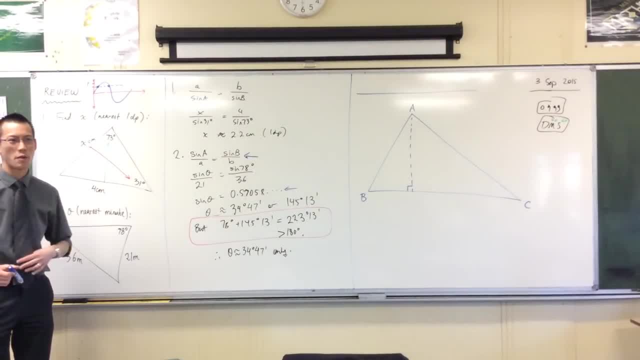 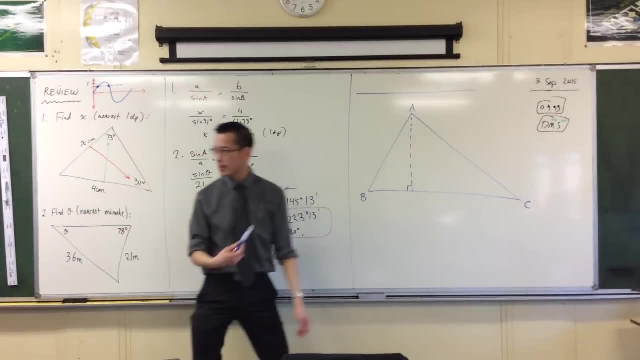 Starts with an A. We tend to talk about planes having this kind of thing. It's the um, It's the altitude, It's an altitude, okay. Also, in this case, it's the perpendicular height of the triangle. So I've got this labeled in. 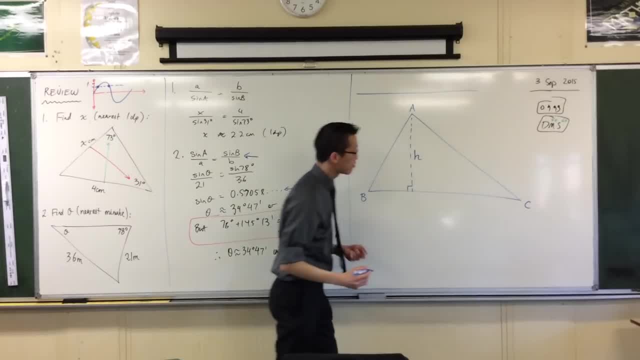 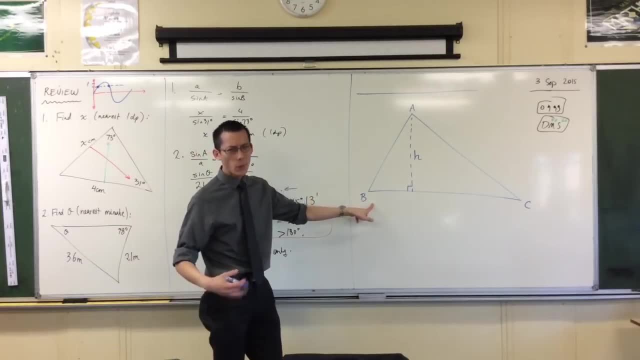 Because it is like the perpendicular height, I'm going to call this h, right? And our conventions for sines and points and how they match up is that, for instance, if this is capital B, what would we usually call this length over here? 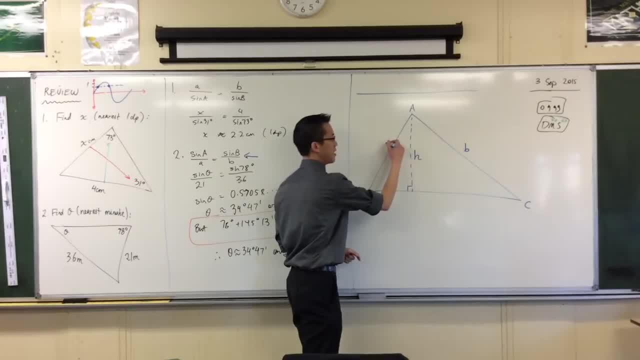 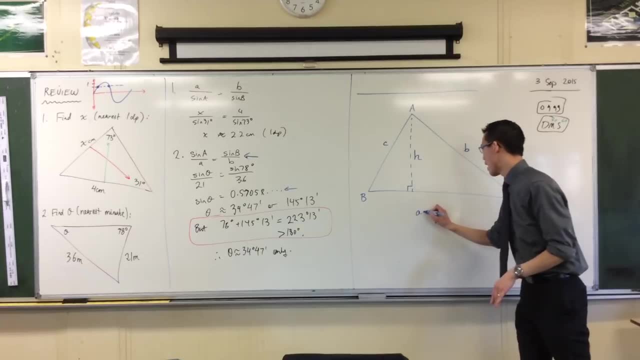 Small b. We call it small b, lowercase b. right, This is going to be lowercase c over here, because it's opposite that sine That makes this lowercase a down the bottom. Now I'm going to write this length just a bit further off, because what I want to put closer in is the side lengths of these two smaller triangles I've made. 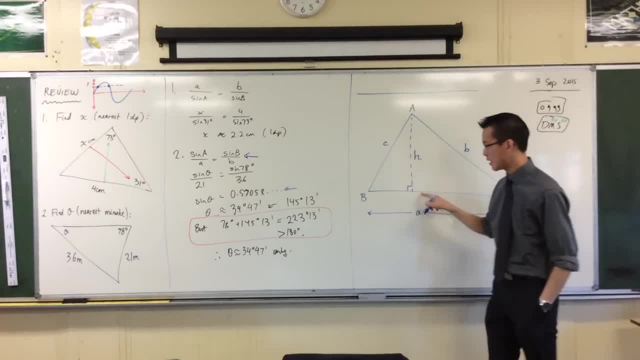 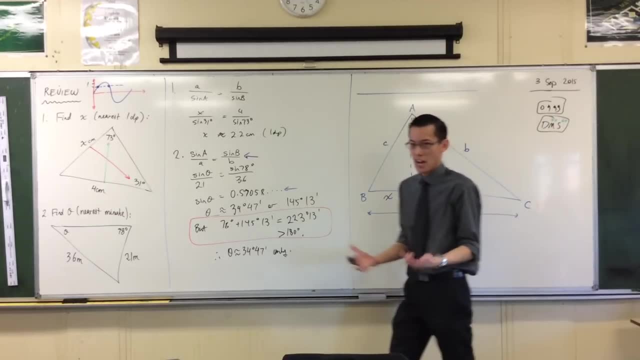 So, just for convenience, I'll call this little length here. from here to that point, we'll call it p for point. I'm going to call b p. I'm going to call that length x, because I don't know what it is. 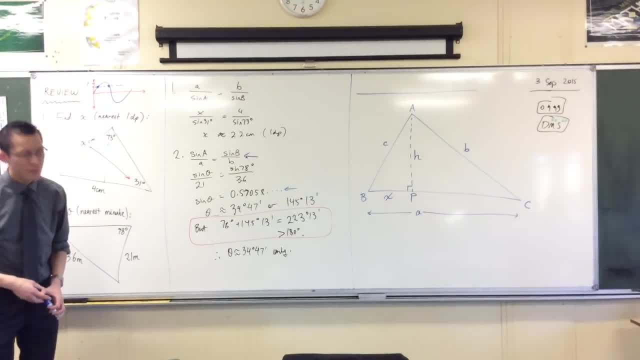 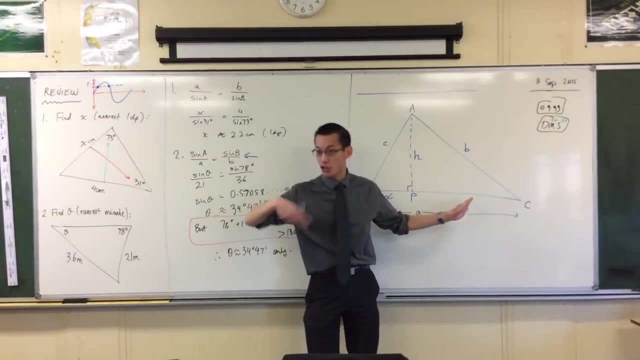 If that little length is x, what's the left over? What is p, c? How long is that One y It's going to be? now I could introduce another letter, but I can phrase it in terms of letters. I already know the pronouns. I already know. 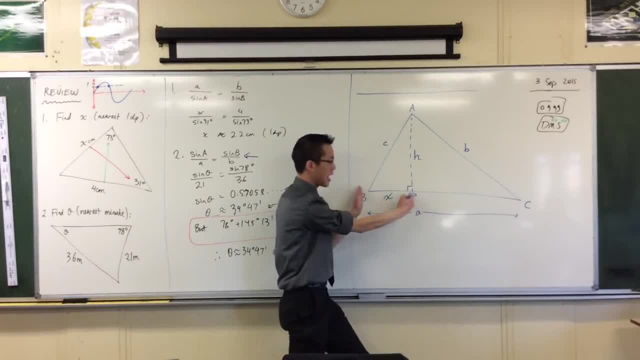 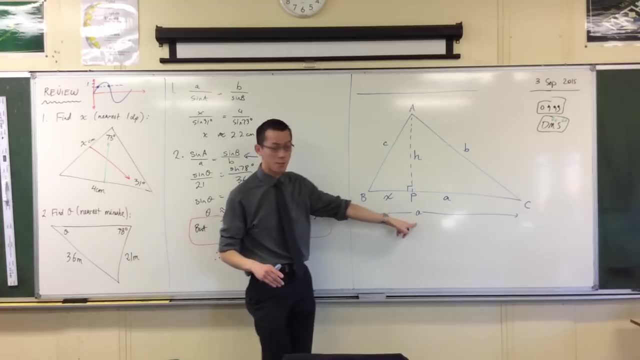 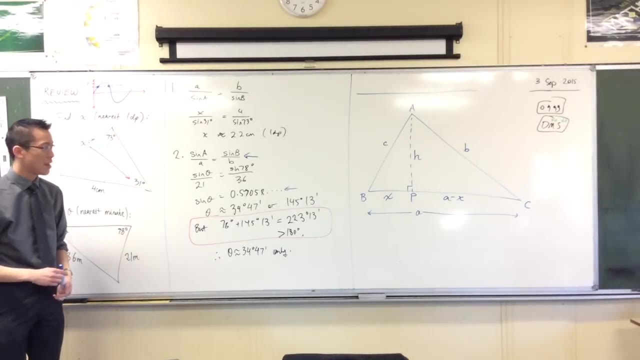 This length is the whole length. a take away this x that I just introduced, So I could say bc or I could just use my lowercase a, and that'll be nice and simple. So are you happy with that? a take away x. 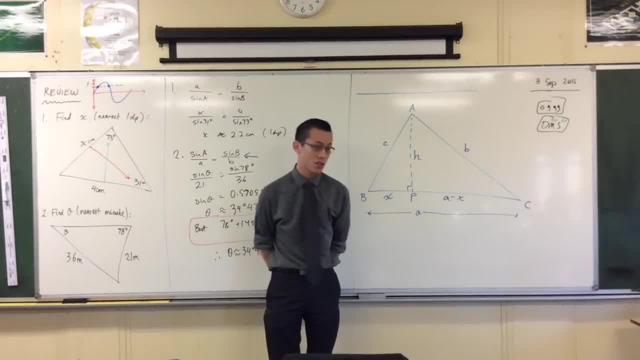 Now we're going to use cosine. Okay, We're going to use cosine instead of sine. but before I reach for that, I notice that because I've got these right-angled triangles, I can use Pythagoras in this pair of triangles as well. 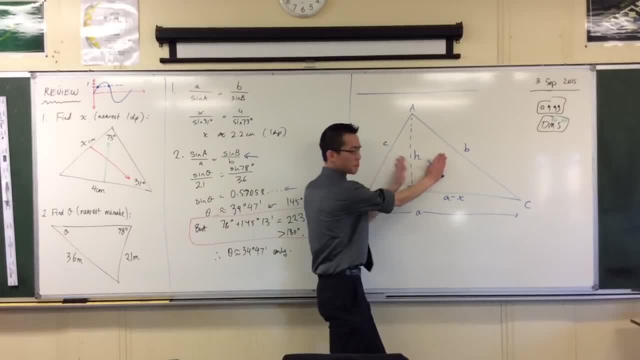 Right, Because h is kind of like the connecting piece between the two triangles. I'm going to say, in this left-hand triangle, in triangle a, b, p, Okay, Through Pythagoras, I can make a statement about h squared. 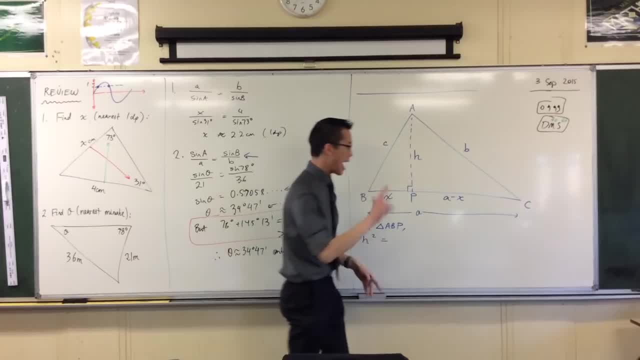 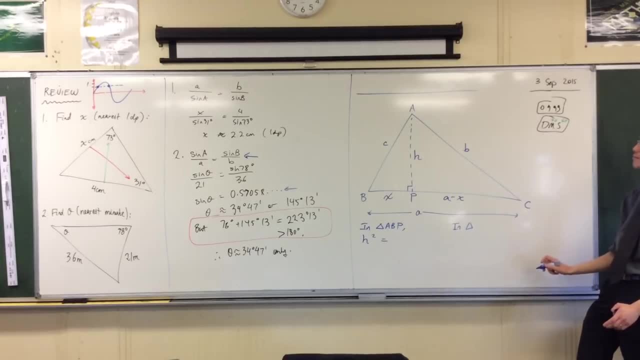 Okay, Like this squared, that squared and this squared Right, And at the same time in this right-hand triangle, I can say: in triangle what's it called? a c p Instead of a b p. 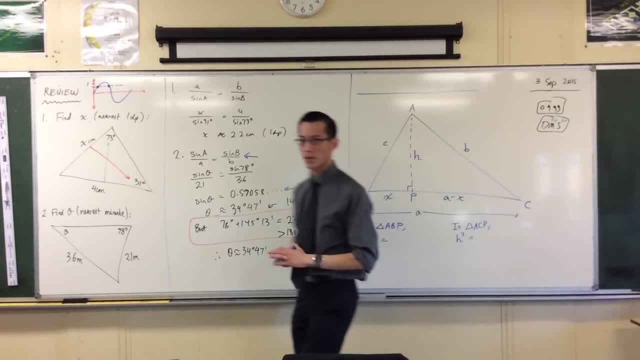 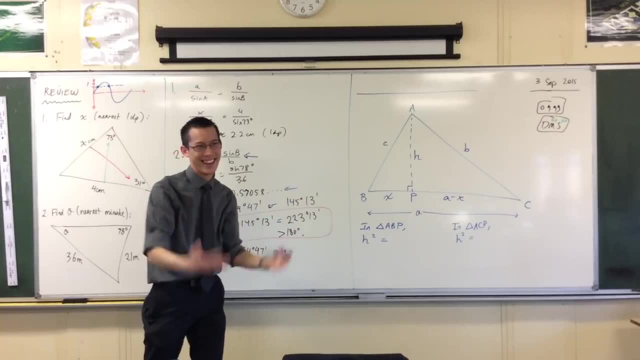 I can say another thing about h squared. Now just to pause, right, Mathematicians do this all the time. They look at the one object and they try and approach it from different angles, literally, Right, Try and get a different perspective on the same thing. 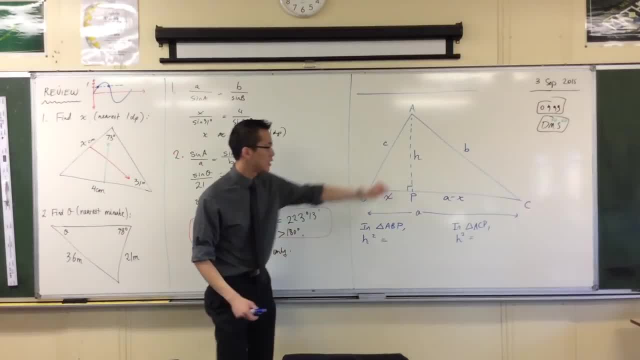 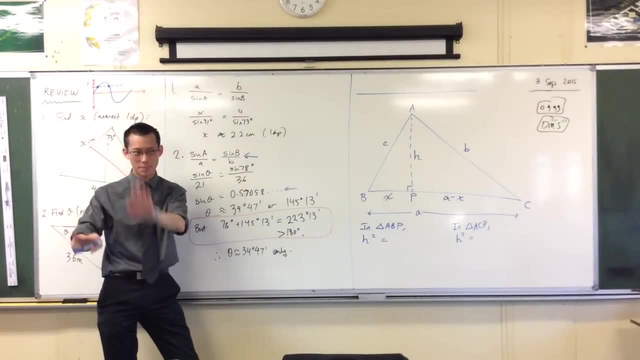 And that tends to yield insight. Right, It's a mathematical thing to do So over here. Right, h squared, it's not the hypotenuse, is it Okay? So I can't say: h squared equals something squared plus something squared, because it's. 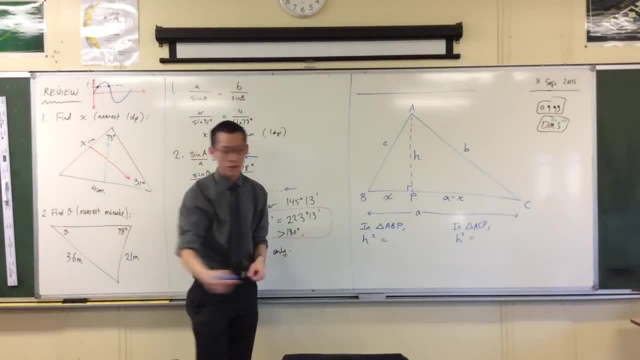 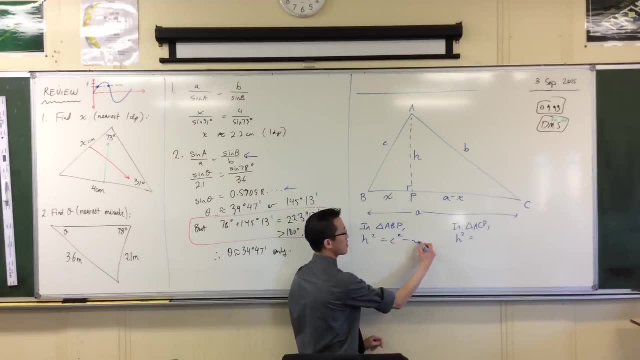 the shortest side. What should I say instead? I'm going to do takeaway Right, So I've got c squared. there's the hypotenuse over here on the left opposite, the right angle: Takeaway x squared. 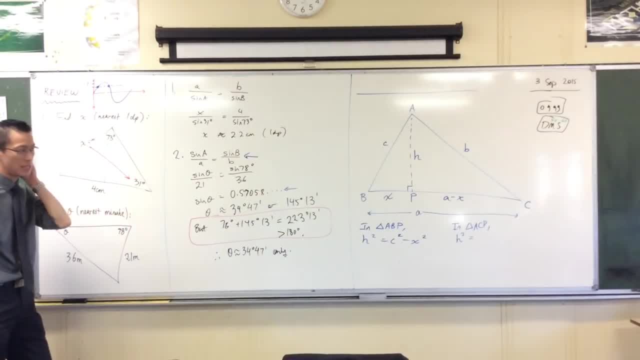 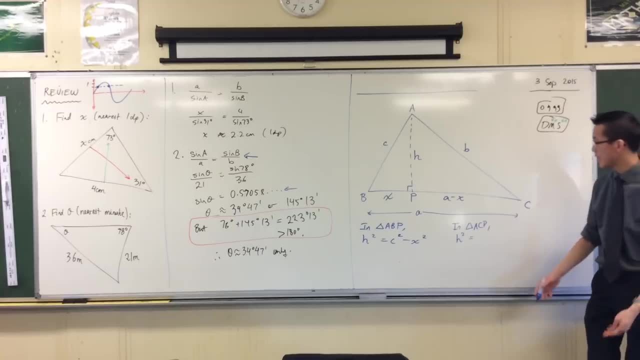 Are you content with that? h squared equals c squared minus x squared, And that's by Pythagoras. It's the implication of Pythagoras. Over here I'll do exactly the same thing, except this is my hypotenuse. 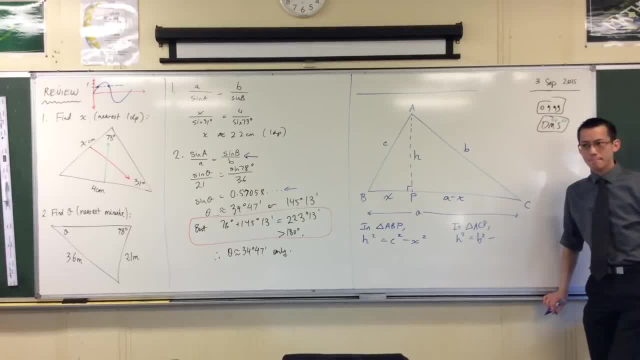 Right, b squared. What am I taking away? Yeah, I've got a minus x and I've got to square that whole thing Right: The whole side, a minus x, that has to be squared. Okay, I need some more space, so bear with me. 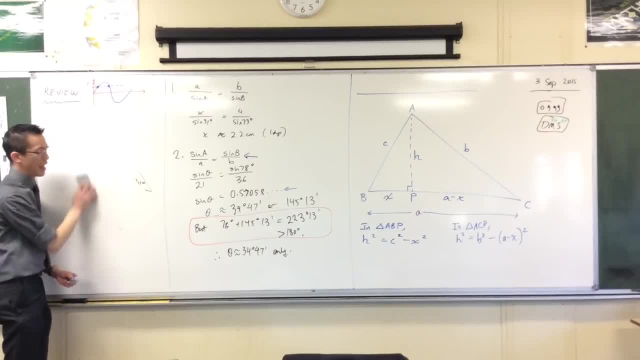 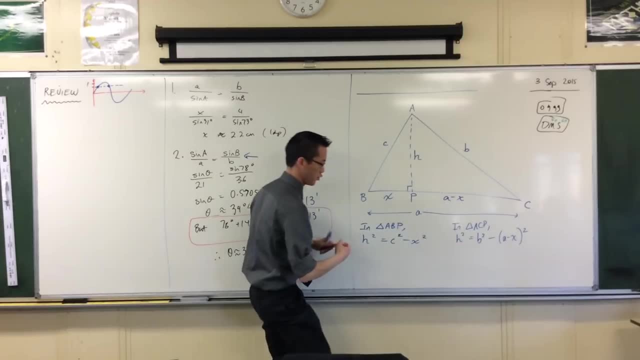 Now that I know what h squared is- and I'm seeing it from two different angles- because it's equal to this, but it's also equal to this- it's pretty reasonable to assume that this and this are really actually equal to each other. 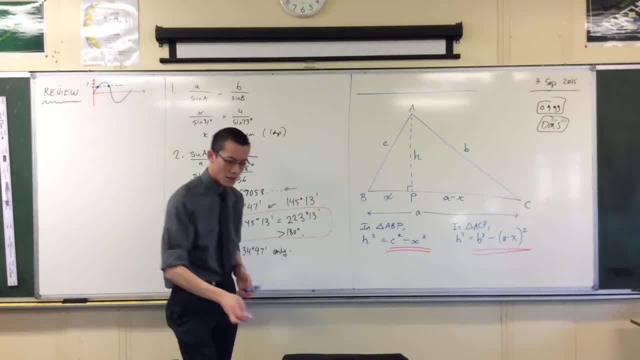 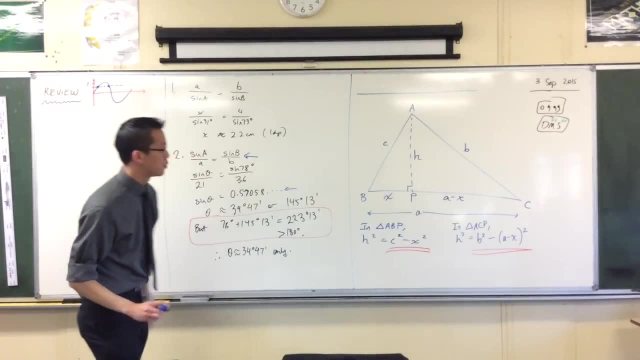 So I can kind of cut out the middle band, as it were. Right? So I can now say, therefore, which side am I going to put? on which side I'm going to put? hmm, which way have I done it? 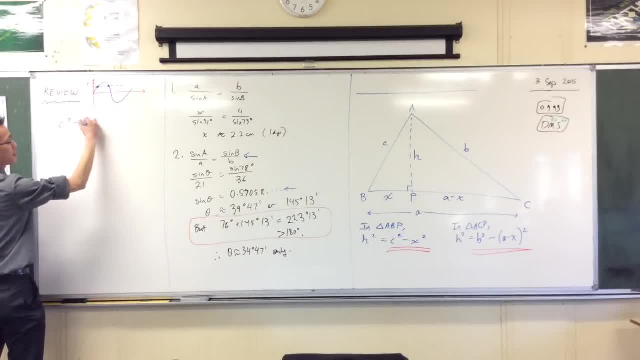 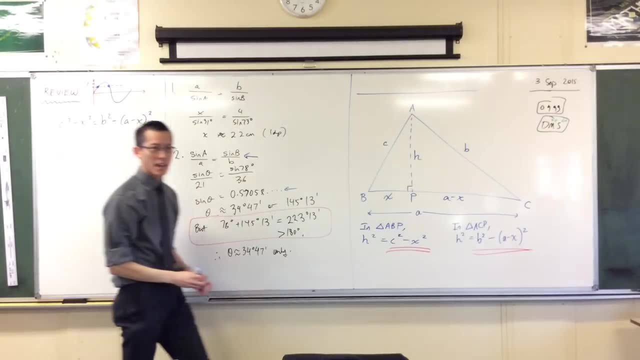 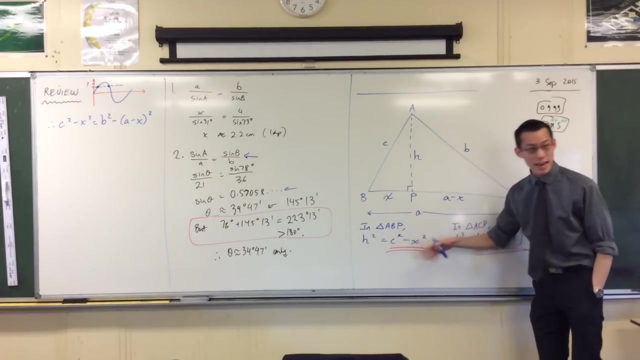 I'm going to put c squared minus x squared. equal x squared equals b squared minus a minus x squared. Are you okay with that? You can see they're both versions of h squared. You can tell with that. so if it's equal to that, and it's equal to that, they should be. 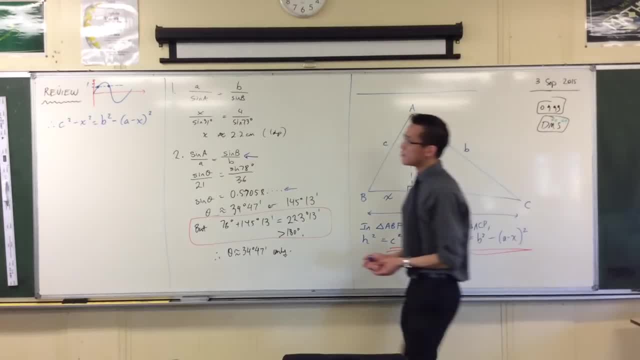 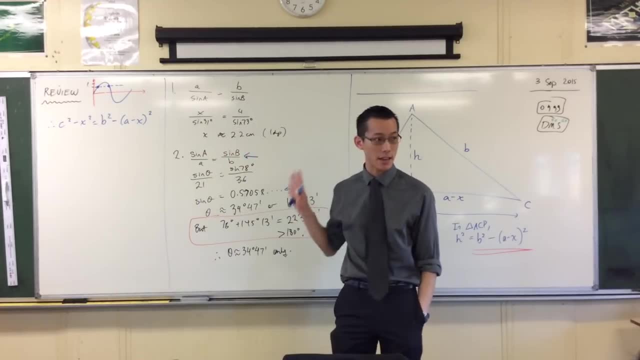 equal to each other. So far, so good. Now, this is true, this is true, but I want to simplify this a little bit, And I know in advance, before I do anything, I should be able to simplify something. Here's how I know. 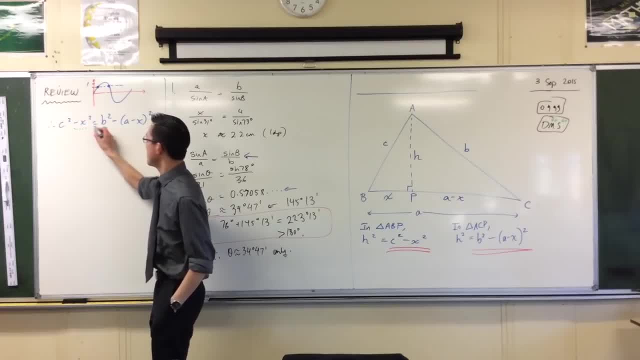 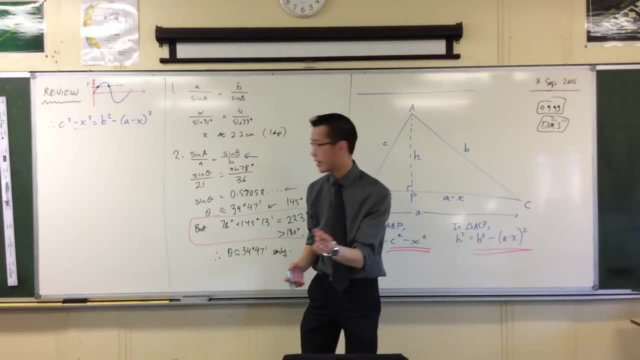 Okay. So when you see there's an x squared there right Or a minus x squared On the right-hand side, there's something I can expand Once. I do it because there's an x and it's being squared right. 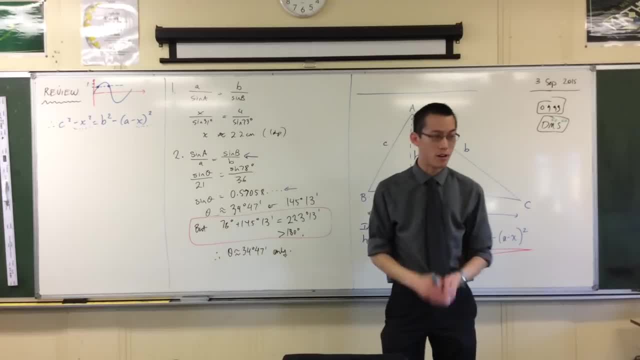 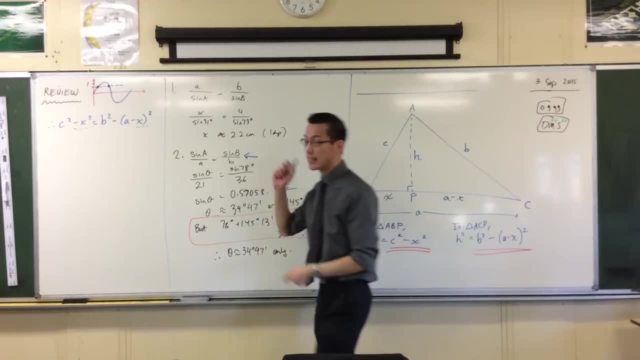 I'm going to expect that there will be a minus x squared on the right-hand side as well. If you've got the same thing on the left as you have on the right, you can get rid of both of them, Okay. So that's kind of what I'm anticipating. 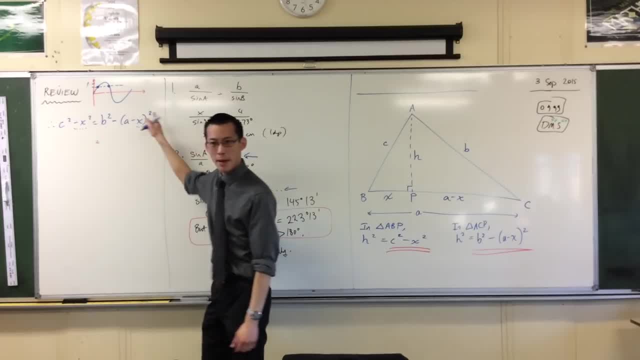 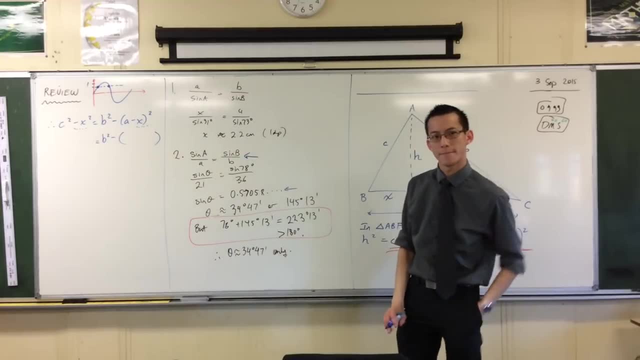 Let's give this a go. There's not much to do on the left-hand side. Let's expand out this right-hand side, though. Okay, B squared. take away What is a minus x? once you're squared, What am I going to get? 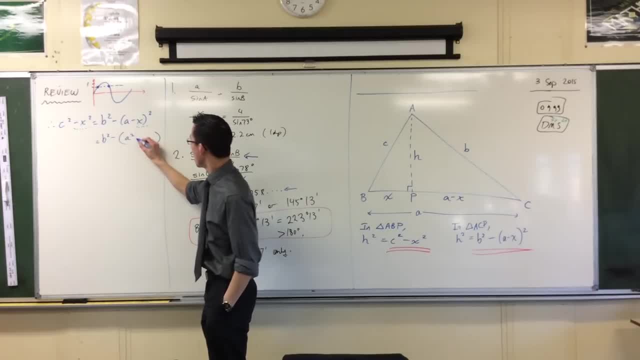 I'm going to get a squared minus 2, 2. what, Excuse me? what? 2ax, 2ax, very good, And then that's okay. That's why we're doing this now. And then you take that x and you square it right. 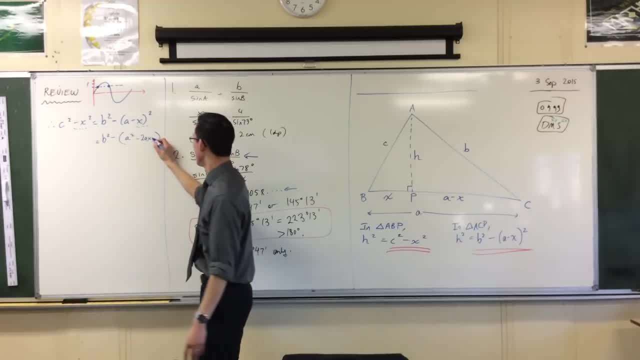 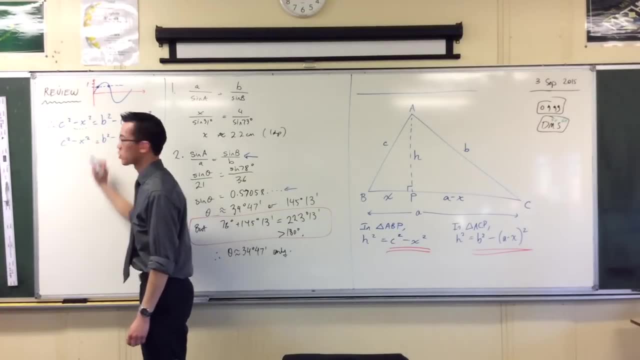 But because it's minus x and it gets squared, the negative disappears, doesn't it? So it's plus x squared. It's a bit small, But you see what I've done, Okay, So I've expanded that And I still have my c squared minus x squared, hanging over there on the left-hand side. 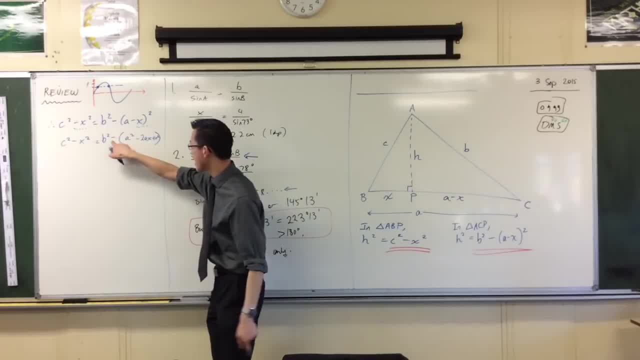 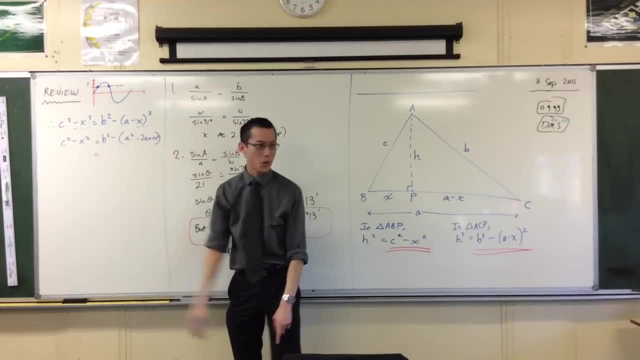 Okay, Now, on the right-hand side, I've got to take away in front of this whole set of brackets. Watch for this. by the way, I could have done this directly in one step, But because doing double negatives is an error that people make all the time, even people who have been doing maths for a long time. 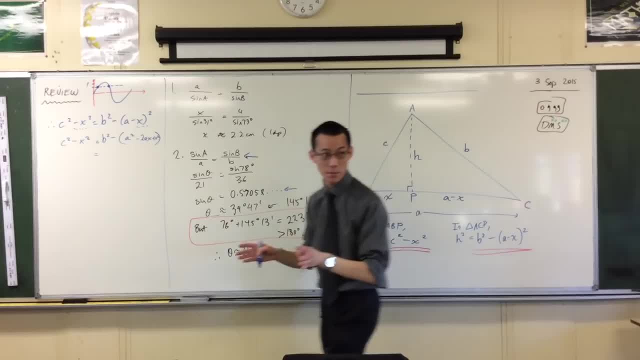 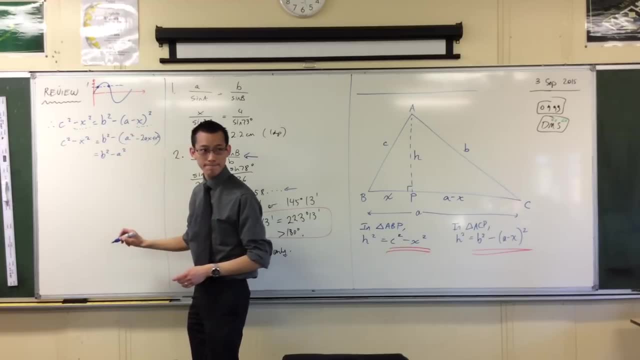 it's worth doing that extra step to make sure we don't accidentally muck something up. So I'm going to do these one at a time, All right? So I've got my c squared minus a squared Double negative there. So plus 2ax. 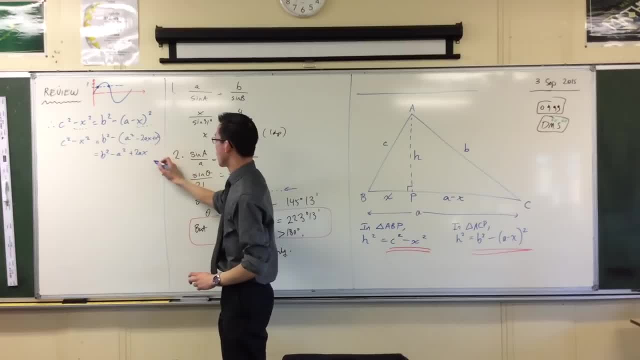 Are you happy with that? Yeah, What am I going to have over here? Minus x squared. Ah, that was the thing I was looking for, Right, Because I have a minus x squared here And I also have a minus x squared there. 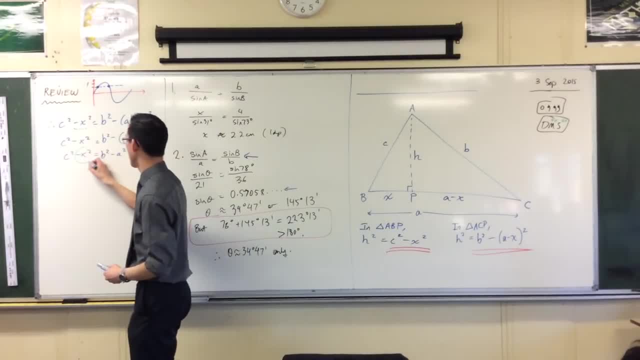 That's really good, Right, Because if I've got the same thing on both sides- 1,, 2, I can get rid of it from both sides. OK, So this is looking good. Now I just have c squared over there. 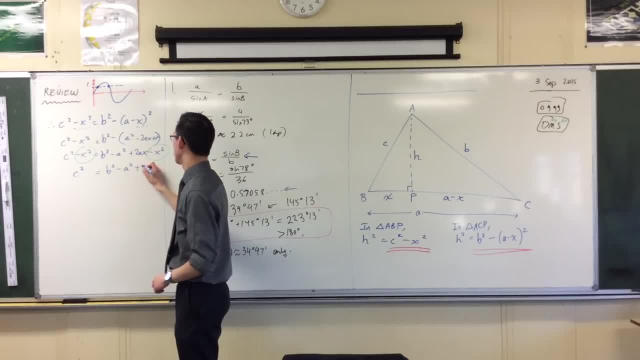 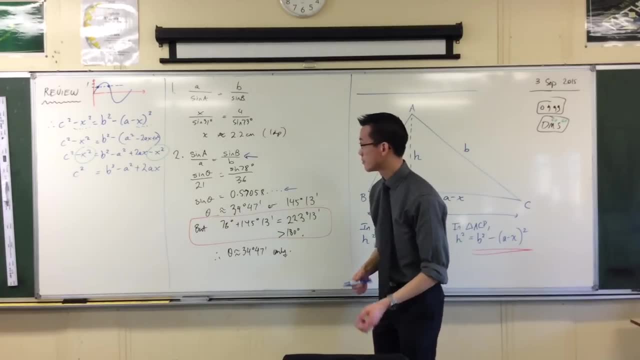 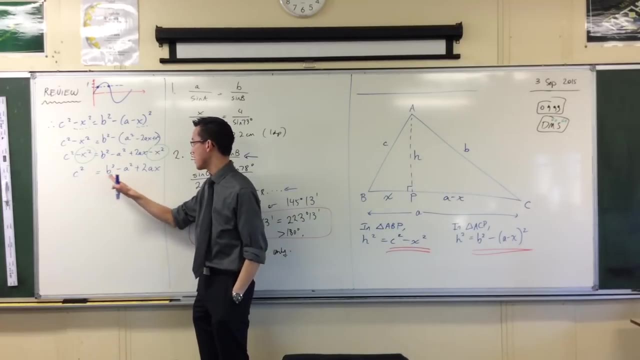 Then I've got b squared minus a squared plus 2ax. Hmm, OK You, happy so far, Happy so far. Things are looking good, OK. Now, what can I do with this? Because I have c, b and a. 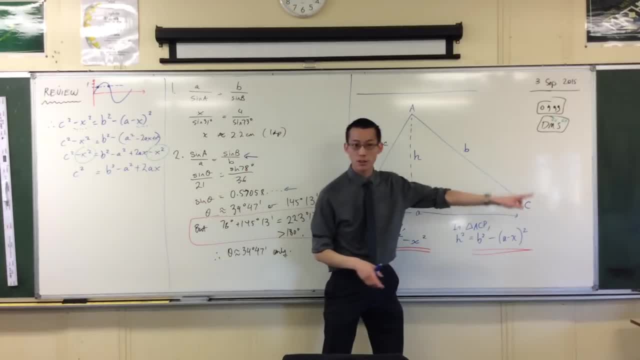 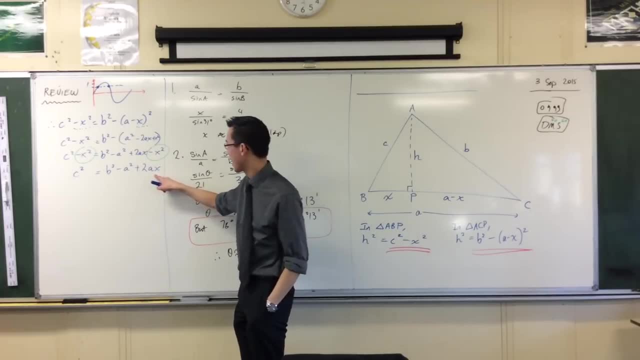 Right, That's really good. They're the three sides of my original triangle, Remember that. But I've got this pesky x hanging around. I don't really want that to be there. OK, I want that to be replaced by something in terms of the a and b and c that I started with. 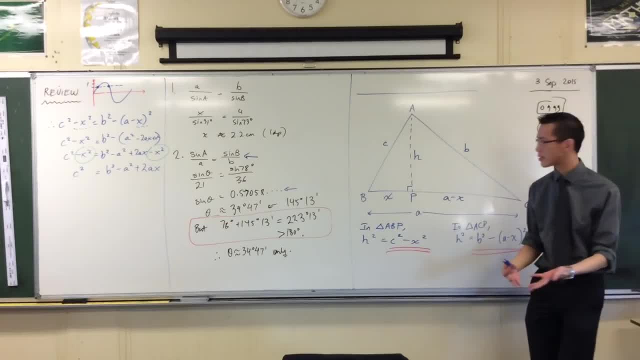 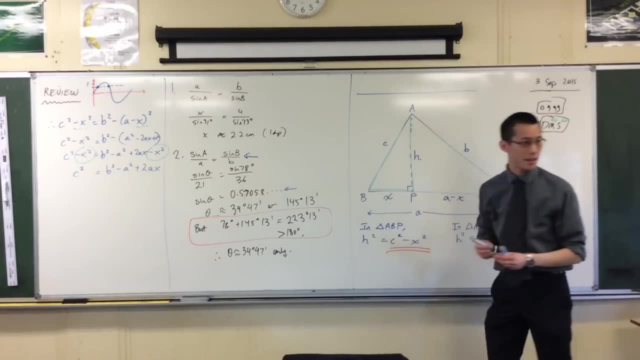 OK. So here's what I'm going to do. Where is x in this diagram? It's in this left-hand triangle. This guy, OK. That guy there, Right? So here's where I'm going to pull cosine in, Right? 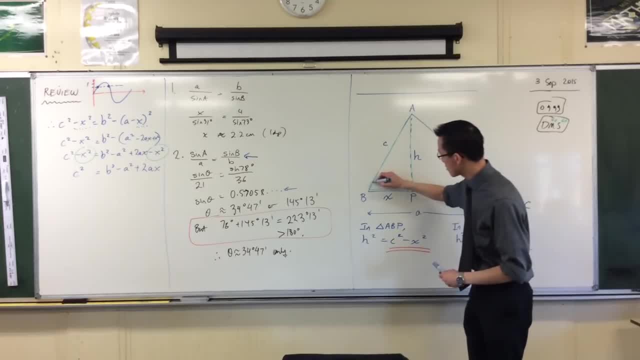 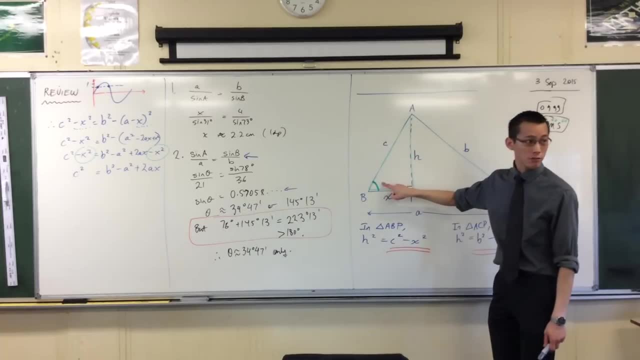 If I say, hmm, how can I get rid of the x? Let's think about things from this point of view. this little angle over here, Right, I could have chosen a different angle if I wanted sine, But this angle is adjacent to x. 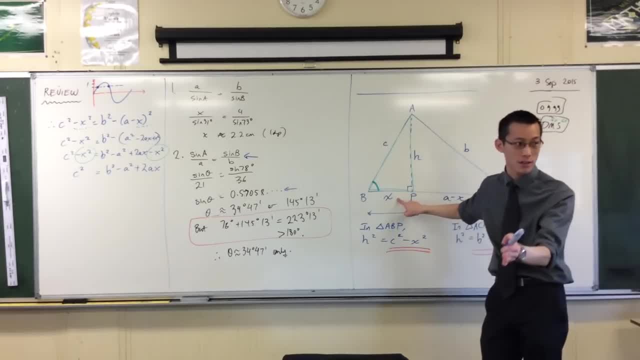 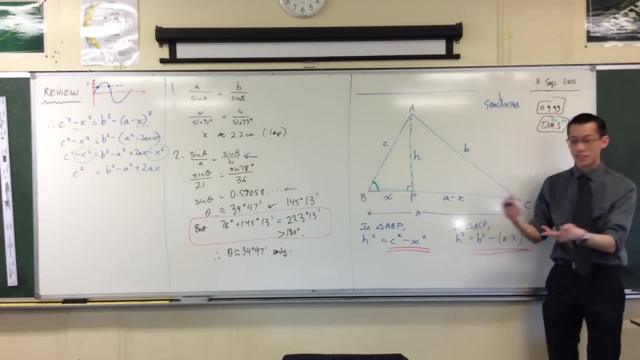 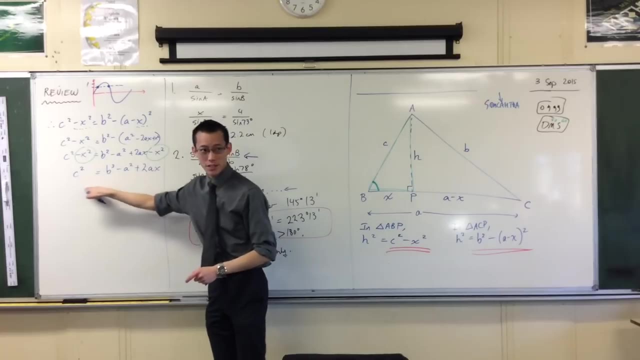 Do you see that It's adjacent, And that's why I go to cosine, Because you remember that cosine is the one which relates the adjacent side to this hypotenuse, which is actually the side of the bigger triangle. OK, So therefore, I'm going to pause this for a second. 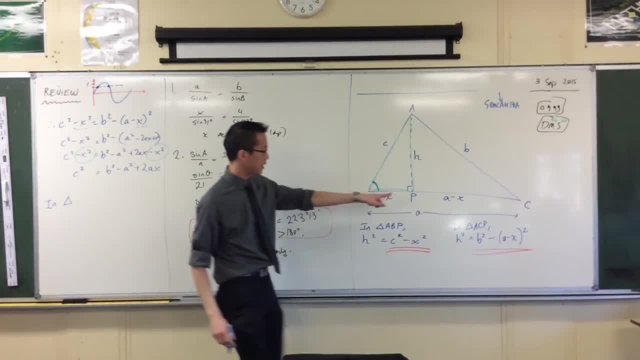 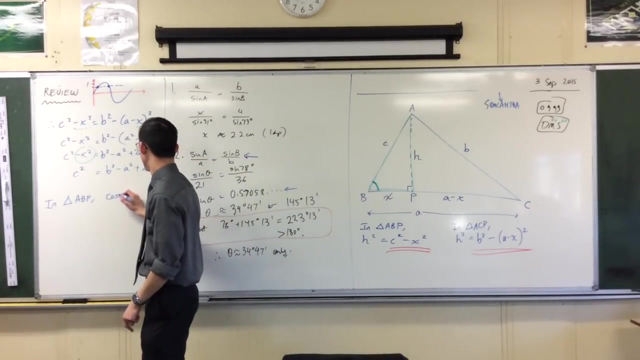 And I'm going to say in triangle. Now have a look, It's this guy over here: a b p In triangle, a b p. I can say cos of this angle over here, cos of b positive b is equal to what's it equal? 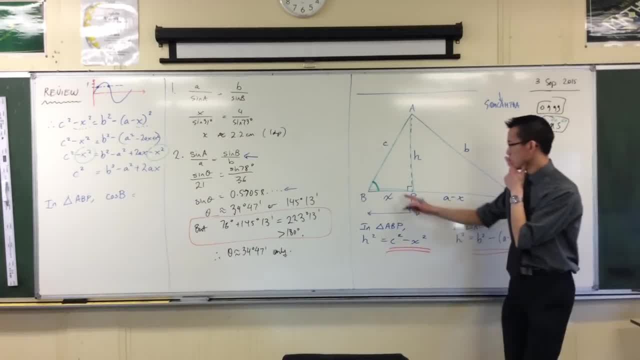 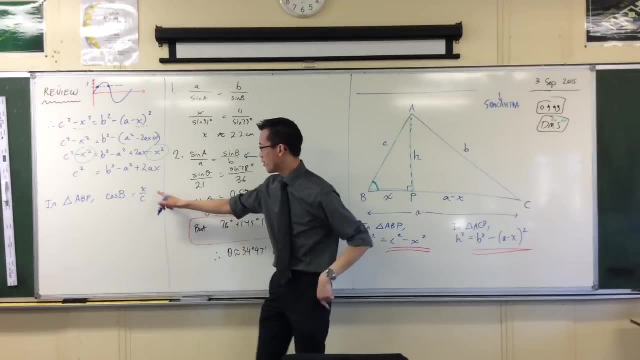 to x over c, x over c adjacent on hypotenuse. Are you happy with that? OK, So now here, I just need to tweak it a little bit to say: well, what's x equal to? Once I've got x equals to something, I can replace whatever that's equal to. 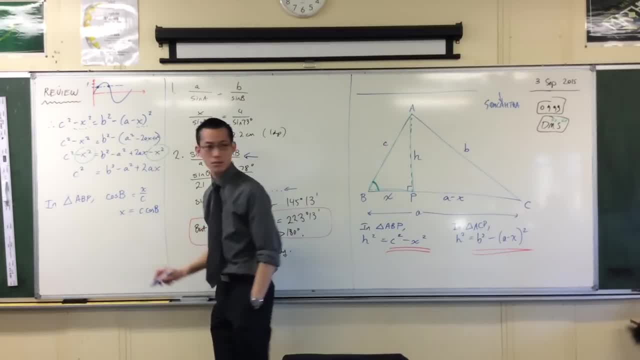 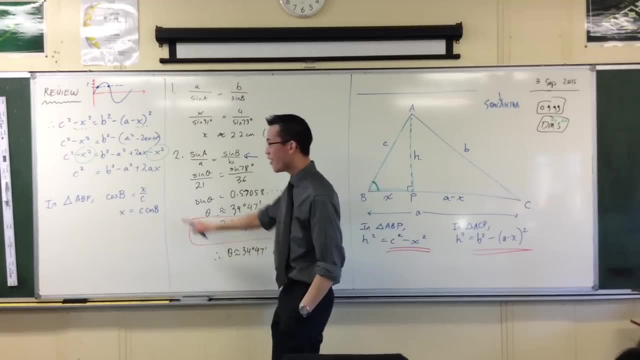 It's going to be c, cos b. Do you see that? I just moved that c over the other side. Don't get freaked out that there are two c's in a row. It's OK. One's a length, One's part of cos. 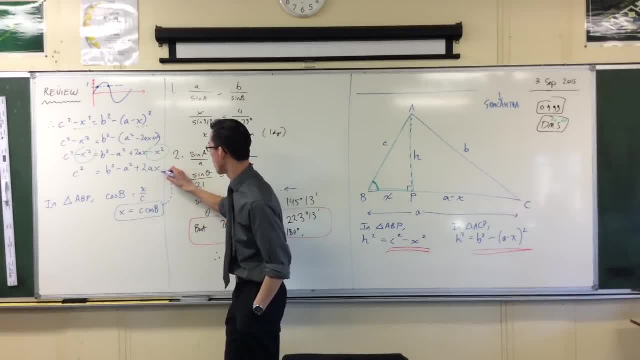 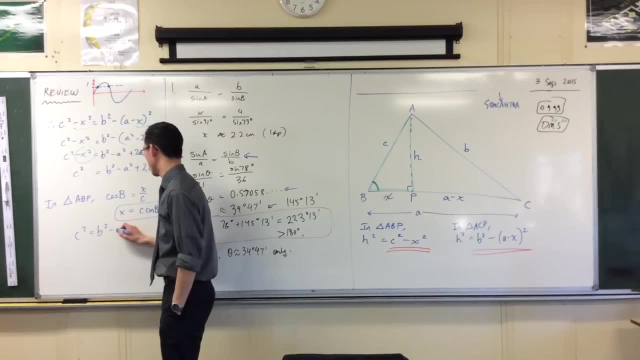 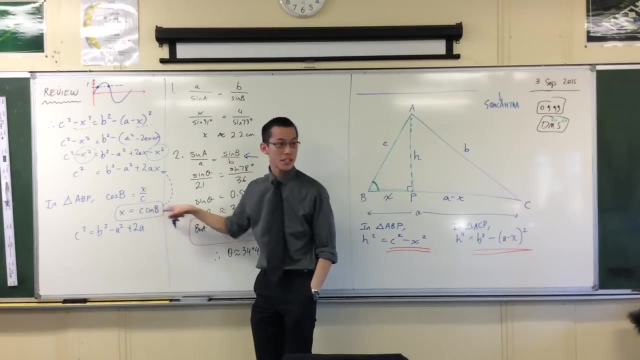 OK, So now this is great, I can use this. I'm going to pop it up into here. OK, So I can say: c squared equals. let's have a look at this: 2a times this guy. This is what I'm replacing x with. 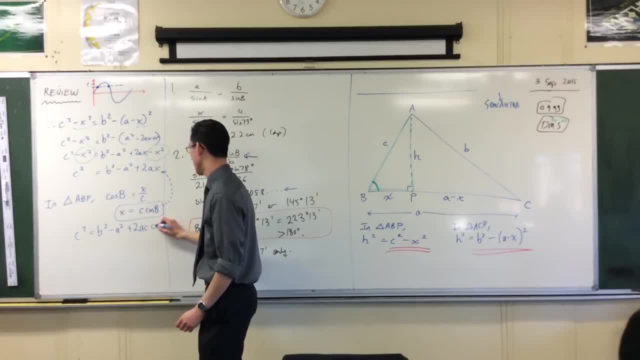 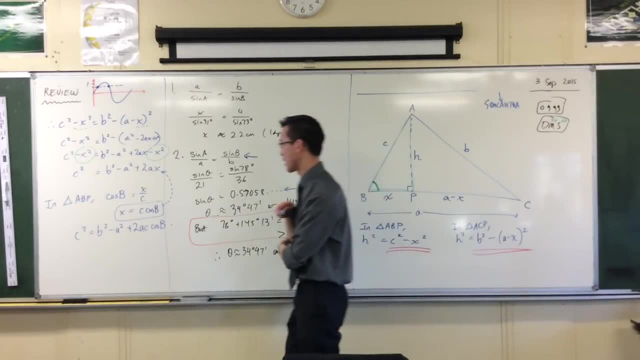 Replacing x with c cos b. I'm going to do one more step to make this nice and clean. OK, I can see c, a, b and c. Right, I could have rearranged them. I could have rotated them any way that I liked. 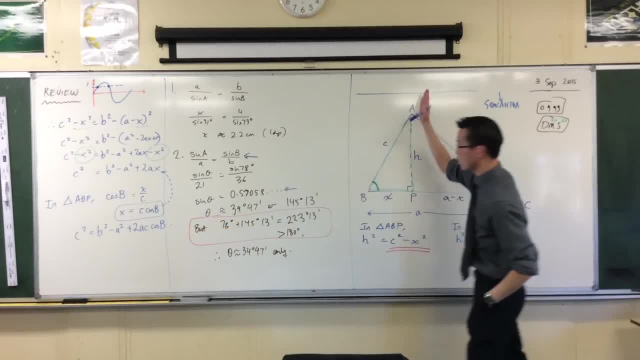 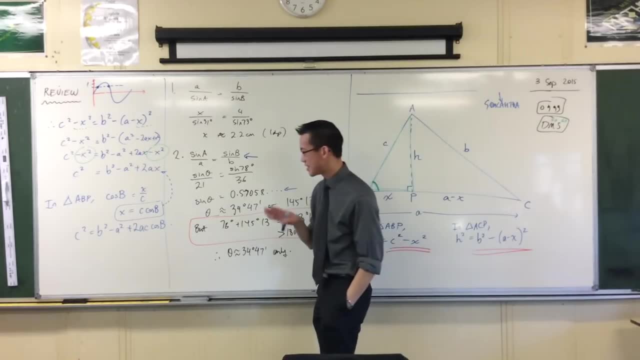 Right, So I could have, for example, instead of drawing this altitude, I could have drawn it that way, or I could have drawn it that way. OK, So I'm going to rearrange the letters ever so slightly Right From this line. I will use red. 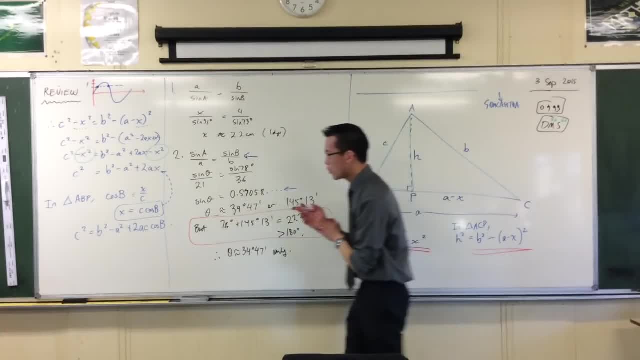 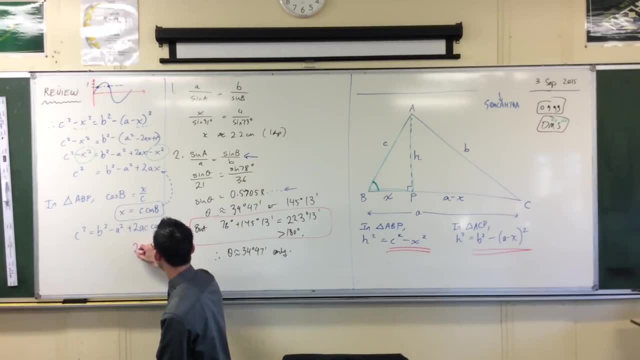 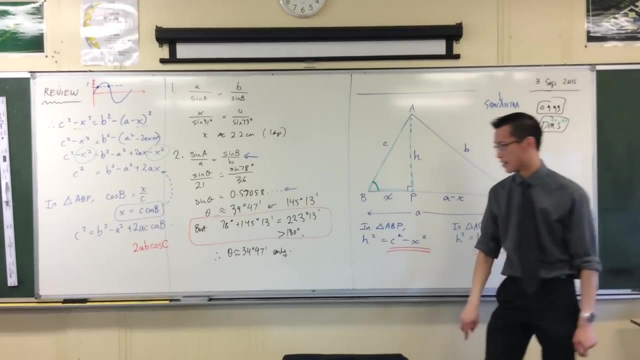 OK. I want to say: OK, here we go. Should I get this right? No, I want this one to be c. What I'm going to do is I'm going to swap b and c around. Everywhere I see a b, I'm going to swap it for a c. 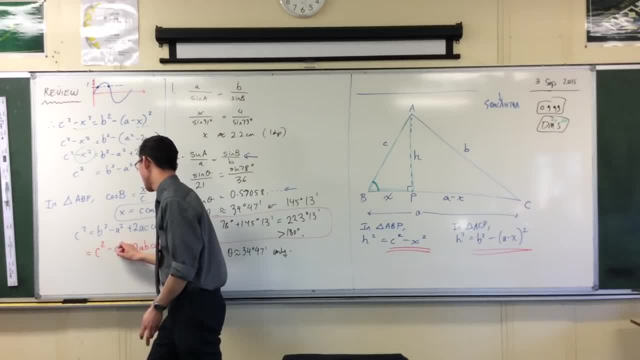 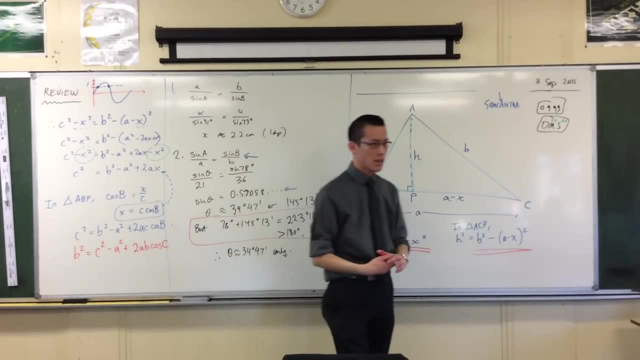 Right, So that gives me a c squared there and a b squared there. Whoops, I missed the plus. OK, So all I've done. it's exactly the same statement, Right? I'm just looking at it from a different angle. 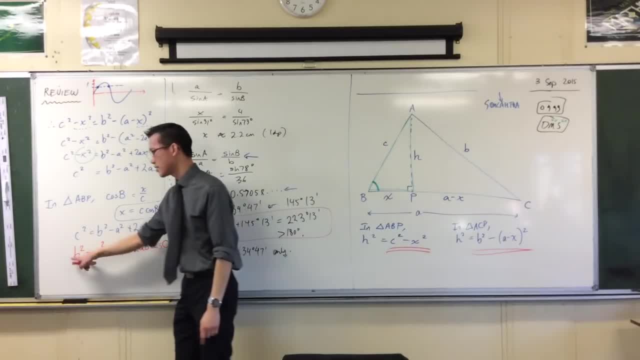 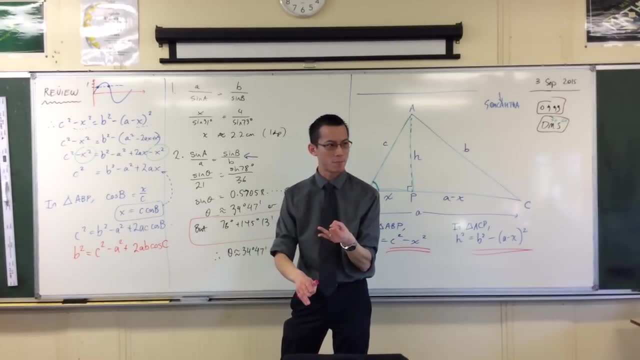 OK, Literally from a different angle. So I've swapped my b's and my c's and they're all fine. OK. Now see how I've got an a squared and a b squared and a c squared Right. We use a squared and b squared and c squared in Pythagoras all the time.